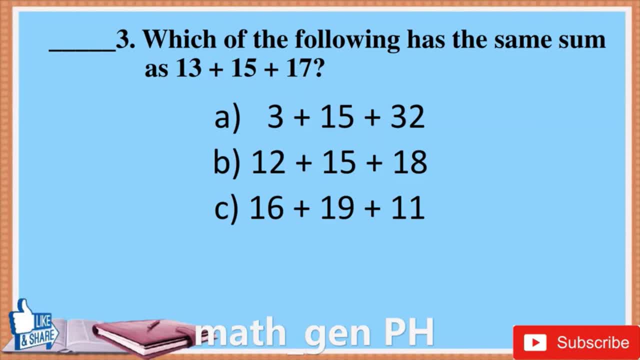 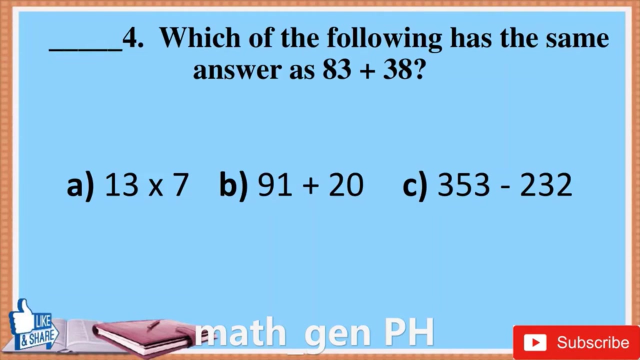 b- 12 plus 15 plus 18.. c- 18. c- 16 plus 19 plus 11. 4. Which of the following has the same answer as 83 plus 38.. a- 13 times 16.. 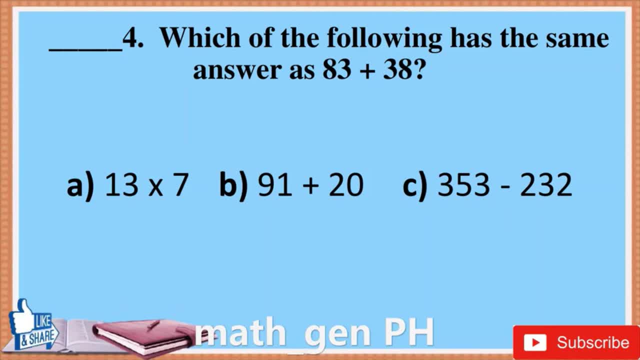 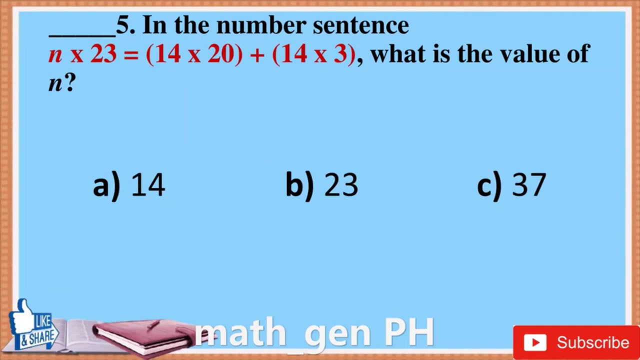 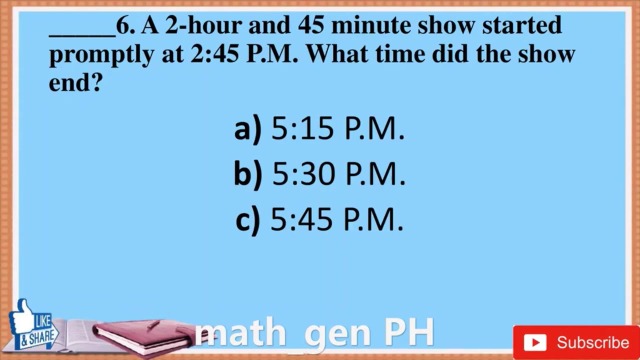 7. B91 plus 20. C353 minus 232.. 7. B91 plus 20. C353 minus 232.. 7. B91 plus 20. C353 minus 232.. What time did the show end? 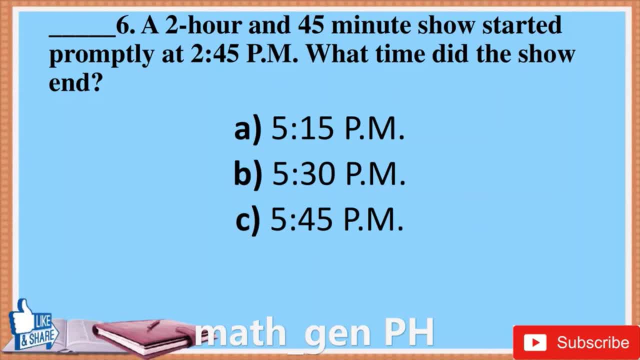 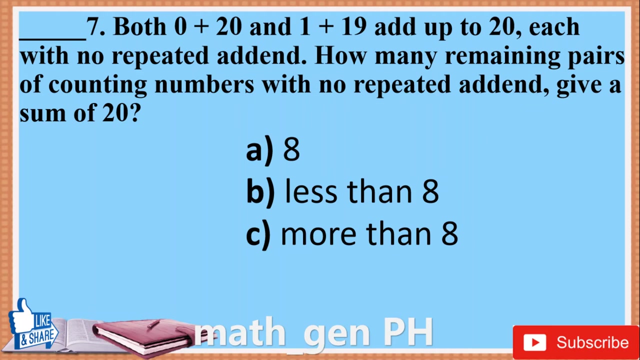 A, 5.15 pm, B, 5.30 pm, C, 5.45 pm, 7. 7. 7. Both 0 plus 20 and 1 plus 19 add up to 20, each, with no repeated add-end. 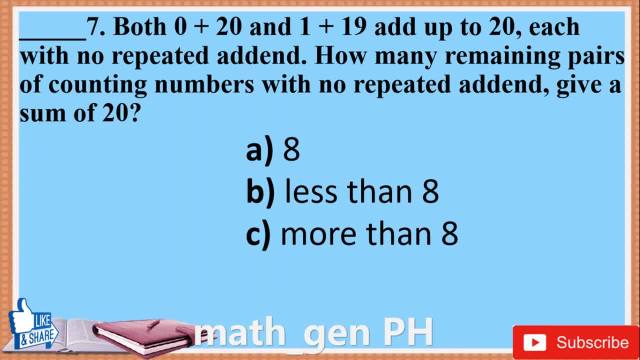 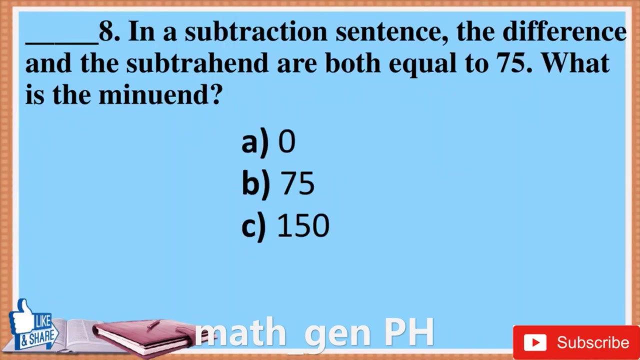 How many remaining pairs of counting numbers with no repeated add-end give a sum of 20?? A- 8. B Less than 8. C More than 8. C Less than 8. 8.. In a subtraction sentence, the difference and the subtrahend are both equal to 75..